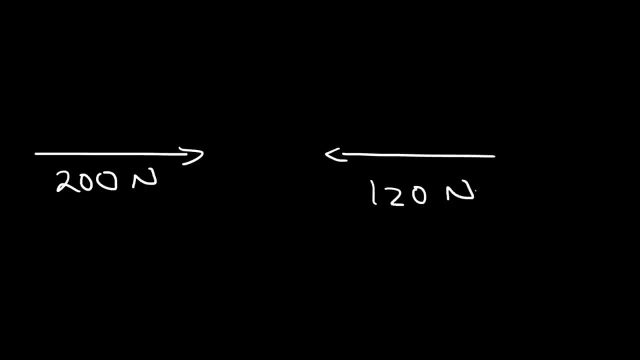 What is the resultant vector and also specified the direction. So this is positive 200 because it's directed towards the right. This is negative 120 because it's directed towards the left. If you add these two, you should get a net force of positive 80.. Now it's going to be smaller than the original. 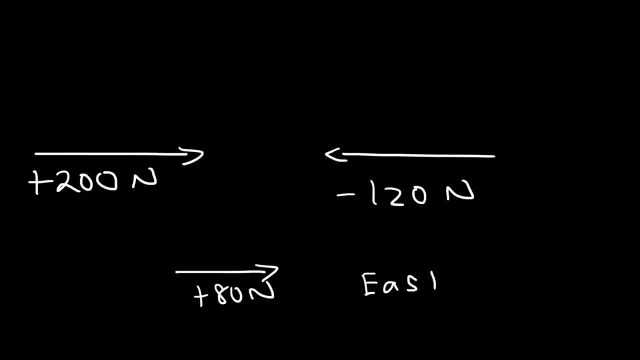 one, but it's still directed east because this vector is greater than this one. Now, as another example, let's say: if we have a force vector that's 60 newtons directed east and another one that's 90 newtons directed west, What is the resultant force vector? and? 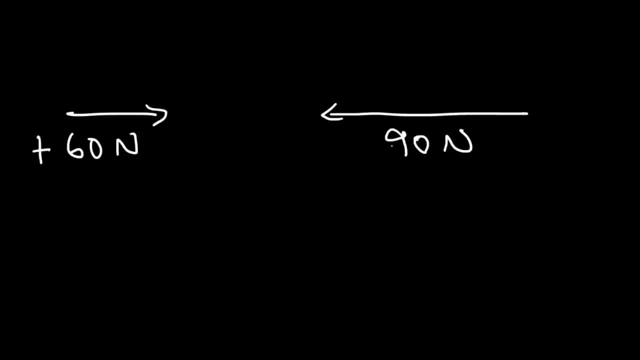 what's the direction? So this is positive 60, that's negative 90. So we're going to have a net force of negative 30 newtons, Or you could just say 30 newtons directed west. Now what if we have a force that's: 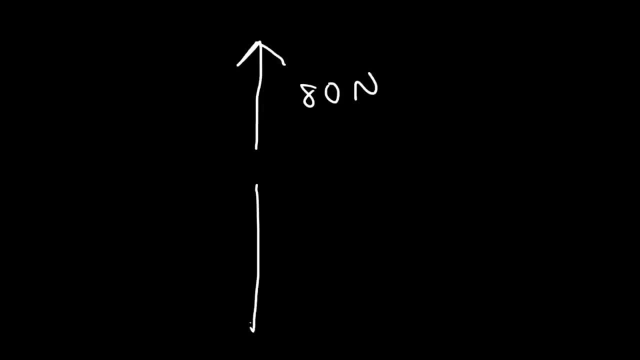 80 newtons directed north and another one that's 120 directed south. So 120 minus 80 is 40. So the net force is going to be 40 directed south And, if you recall, this is north, south, east, west. 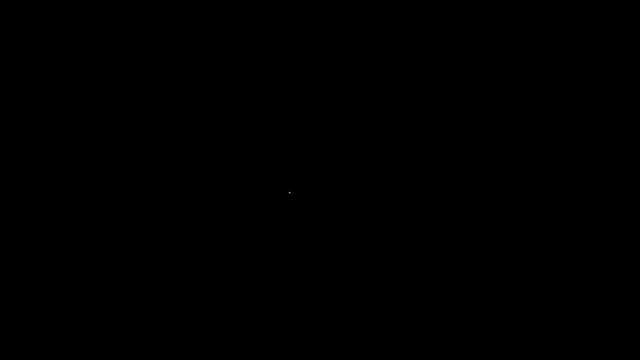 Now, sometimes you may need to add two vectors that are not parallel or anti-parallel to each other. So let's say, if we have a 30 newton force vector directed east and a 40 newton force vector directed north, what is the resultant force vector If you have two vectors that are perpendicular to each other? 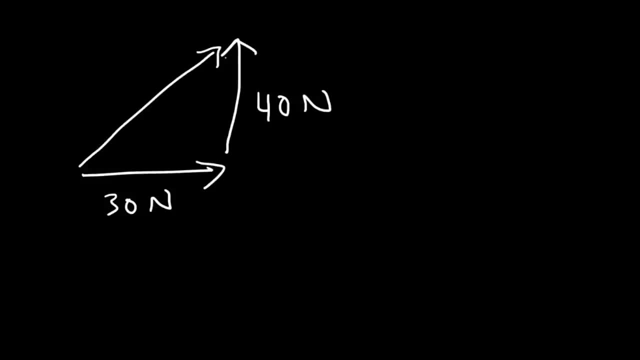 you could find the resultant force vector by finding the left of the hypotenuse of the right triangle that is formed. So therefore, the resultant force vector is: the resultant force vector is going to be the square root of F1 squared plus F2 squared. 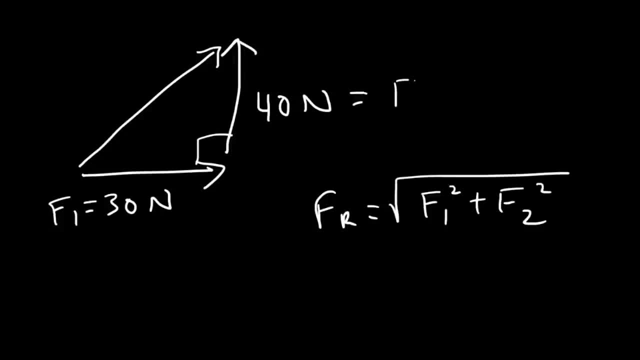 Let's call this F1 and this force F2.. So it's going to be the square root of 30 squared plus 40 squared. If you're familiar with the 3-4-5 triangle, then this is going to be the 30-40-50 triangle. 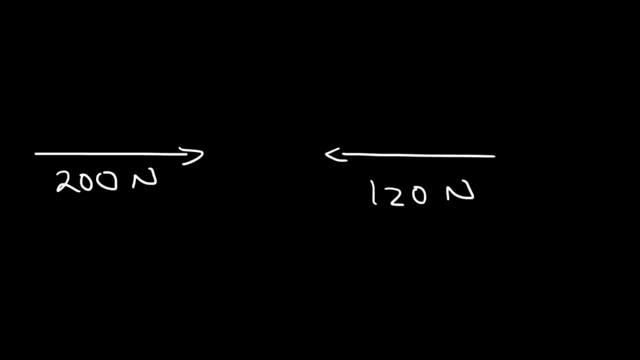 What is the resultant vector and also specified the direction. So this is positive 200 because it's directed towards the right. This is negative 120 because it's directed towards the left. If you add these two, you should get a net force of positive 80.. Now it's going to be smaller than the original. 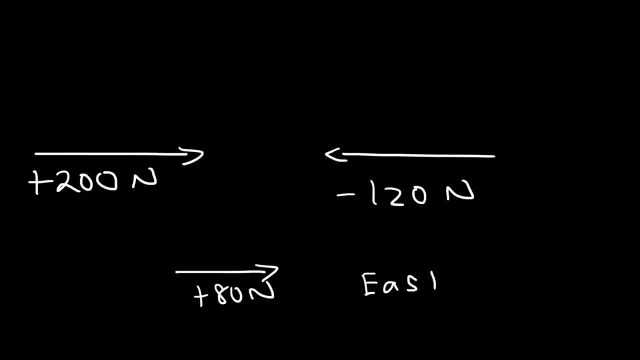 one, but it's still directed east because this vector is greater than this one. Now, as another example, let's say: if we have a force vector that's 60 newtons directed east and another one that's 90 newtons directed west, What is the resultant force vector? and? 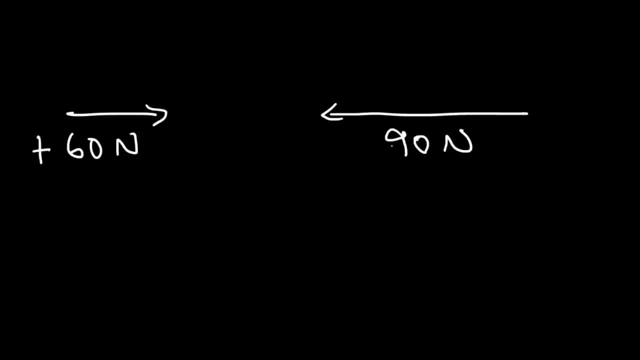 what's the direction? So this is positive 60, that's negative 90. So we're going to have a net force of negative 30 newtons, Or you could just say 30 newtons directed west. Now what if we have a force that's: 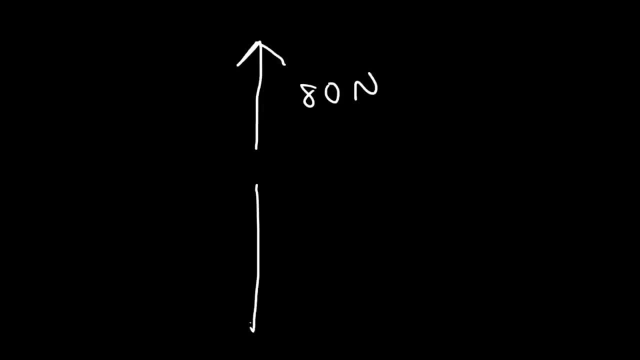 80 newtons directed north and another one that's 120 directed south. So 120 minus 80 is 40. So the net force is going to be 40 directed south And, if you recall, this is north, south, east, west. 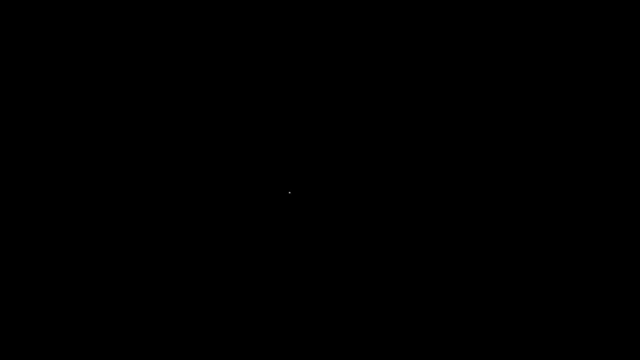 Now, sometimes you may need to add two vectors that are not parallel or anti-parallel to each other. So let's say, if we have a 30 newton force vector directed east and a 40 newton force vector directed north, What is the resultant force vector If you have two vectors that are perpendicular to each other? 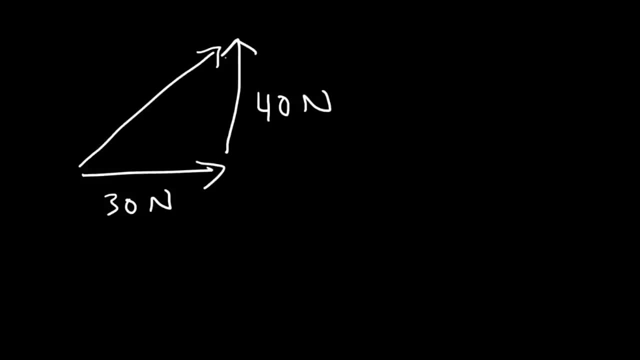 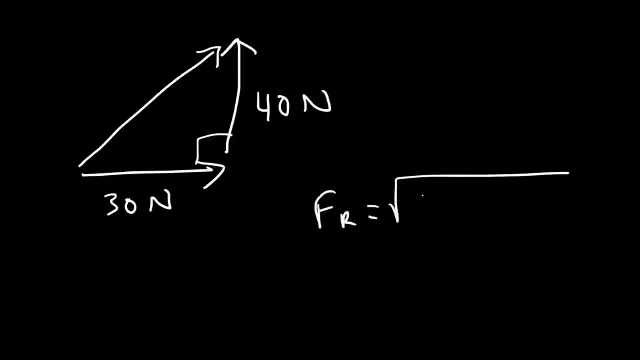 So therefore, the resultant force vector is the resultant force vector. So therefore, the resultant force vector is the resultant force vector is going to be the square root of F1 squared plus F2 squared. Let's call this F1 and this force F2.. 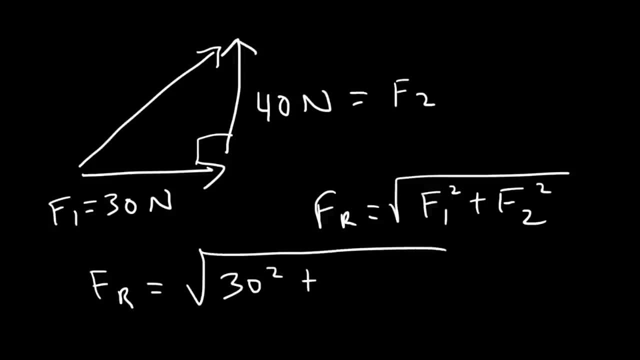 So it's going to be the square root of 30 squared plus 40 squared. If you're familiar with the 3-4-5 triangle, then this is going to be the 30-40-50 triangle, So the resultant force is going to be 50 newtons. 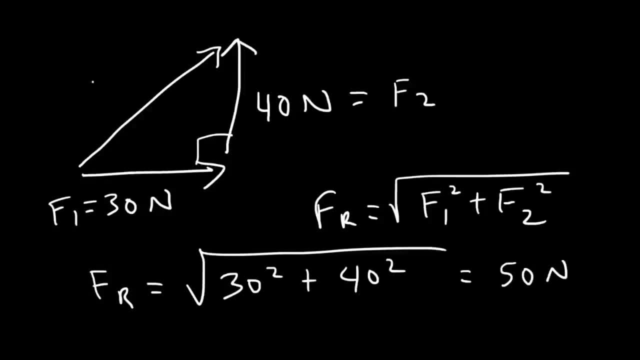 So the resultant force is going to be 50 newtons. Now sometimes, in addition to finding the magnitude of the resultant force vector, which is 50, you may need to find the direction as well. So you've got to find the angle theta. 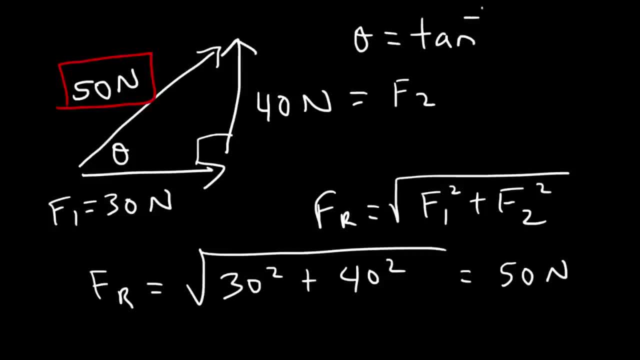 To find it you can use this formula: It's the inverse tangent of the y component divided by the x component. So the force in the y direction is 40, and the x direction is 30. So to find the angle it's going to be: 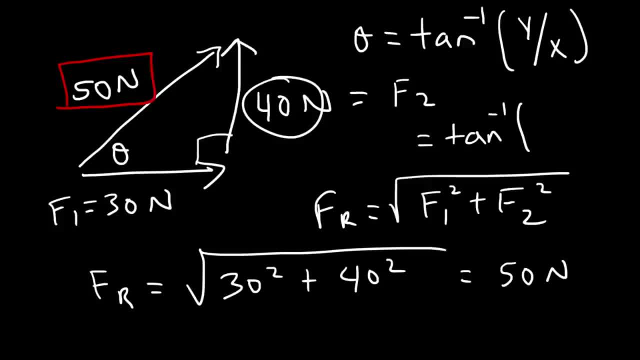 The arc tangent the opposite side, which is the y value of 40, over the adjacent side, which is the x value of 30.. Hopefully you're familiar with SOHCAHTOA. Sine is opposite over hypotenuse, Cosine is adjacent over hypotenuse. 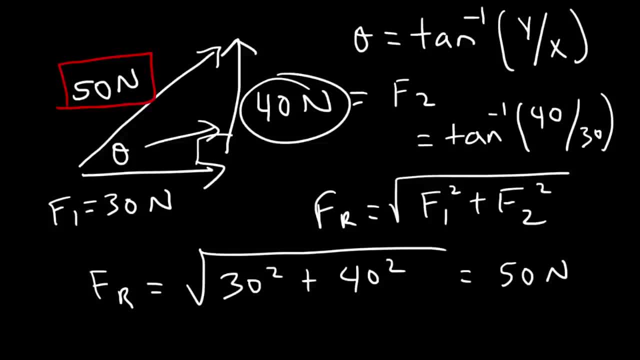 And tangent is opposite. relative to theta over the adjacent side, The arc tangent of 40 over 30 is 53.1 degrees. So we can say that the resultant force vector has a magnitude of 50 newtons and a direction of 53.1 degrees relative to the x-axis. 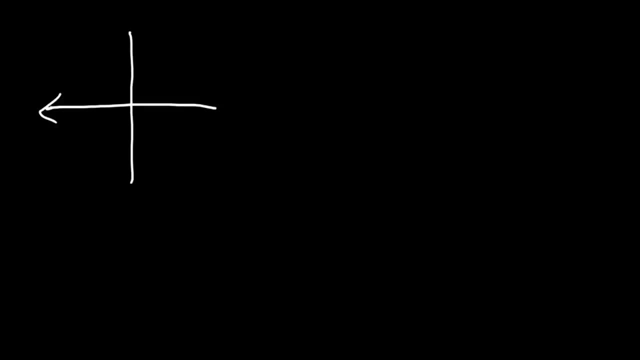 Let's try another example. So let's say, if we have a force vector that's 50 newtons directed west and another one that's 120 newtons directed south, Calculate the magnitude of the resultant force vector and find the direction. 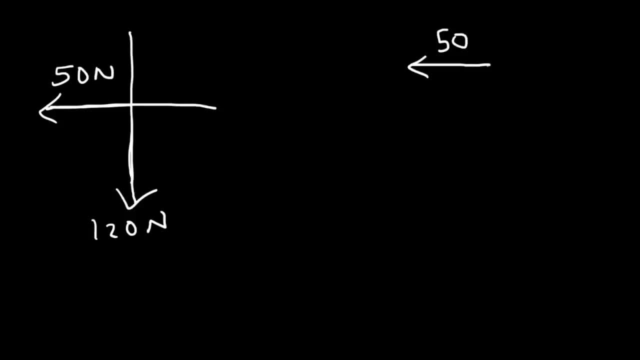 So let's draw a triangle. So this side is 50, and this side is going to be 120. So the resultant force vector is the hypotenuse of this triangle. So notice that it's in quadrant 3.. Now, if you're familiar with the 5-12-13 triangle, 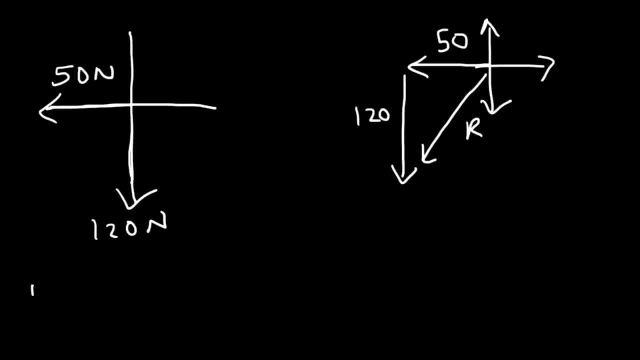 then the hypotenuse has to be 130.. So the resultant force vector is going to be the square root of 50 squared plus 120 squared, And that's going to turn out to be 130 newtons. So that's the magnitude of the resultant force vector. 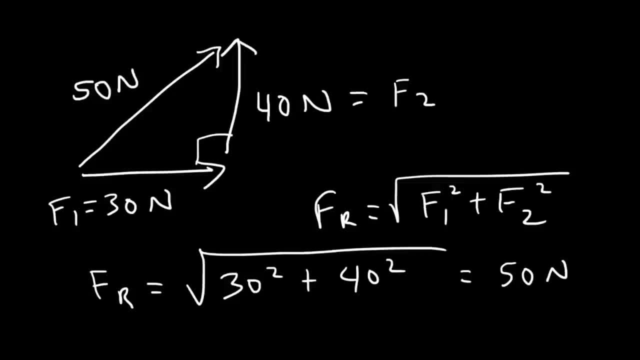 Now, sometimes, in addition to finding the magnitude of the resultant force vector, which is 50,, you may need to find the direction as well. So you've got to find the angle theta. To find it, you can use this formula: It's the inverse tangent of the y component divided by the x component. 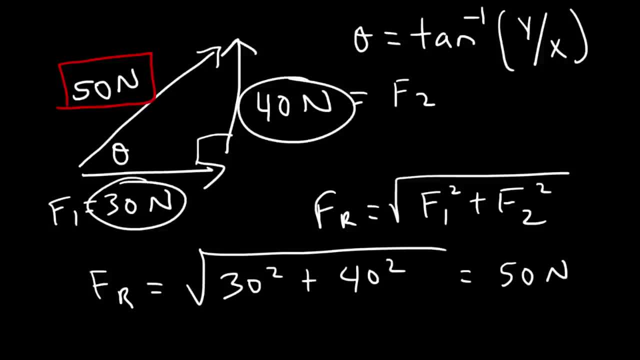 So the force in the y direction is 40, and the x direction is 30. So to find the angle, it's going to be The arc tangent, the opposite side, which is the y value of 40 over the adjacent side. 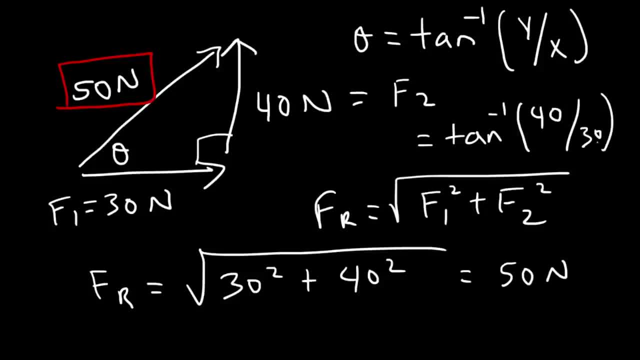 which is the x value of 30. Hopefully you're familiar with SOHCAHTOA. Sine is opposite over hypotenuse, Cosine is adjacent over hypotenuse And tangent is opposite relative to theta. over the adjacent side, The arc tangent of 40 over 30 is 53.1 degrees. 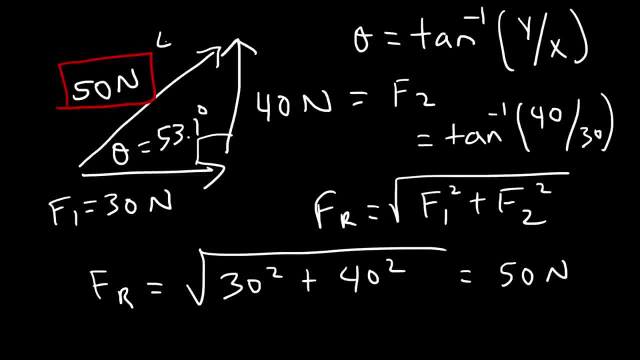 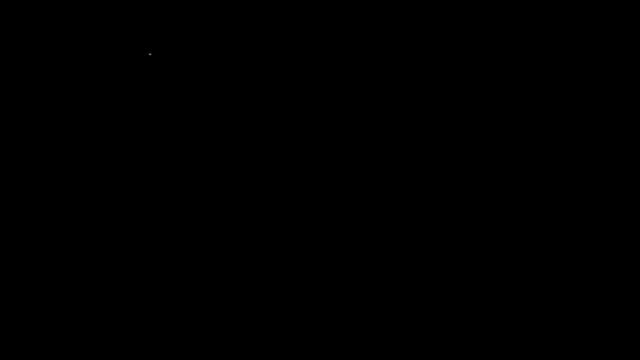 So we can say that the resultant force vector has a magnitude of 50 newtons and a direction of 53.1 degrees relative to the x-axis. Let's try another example. So let's say, if we have a force vector that's 50 newtons directed west, 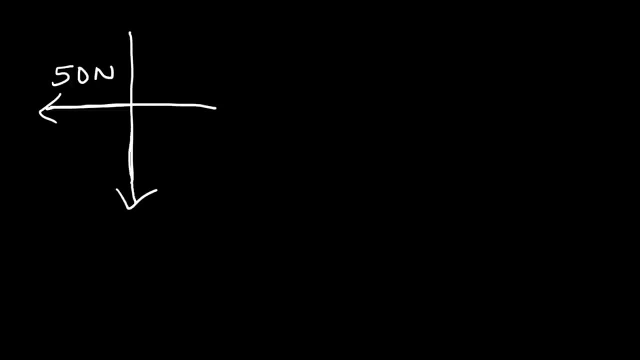 and another one that's 120 newtons directed south. Calculate the magnitude of the resultant force vector and find the direction. So let's draw a triangle. So this side is 50, and this side is going to be 120.. So the resultant force vector is the hypotenuse of this triangle. 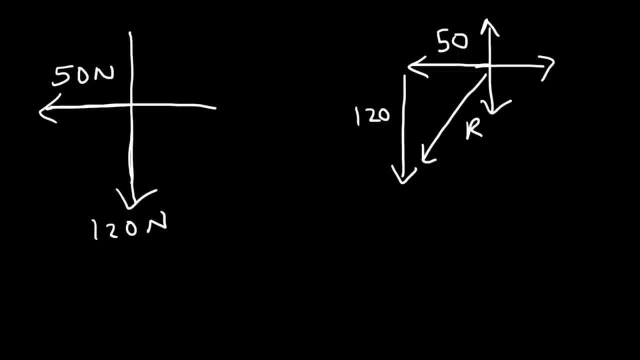 So notice that it's in quadrant 3.. Now, if you're familiar with the 5-12-13 triangle, then the hypotenuse has to be 130.. So the resultant force vector is going to be the square root of 50 squared plus 120 squared. 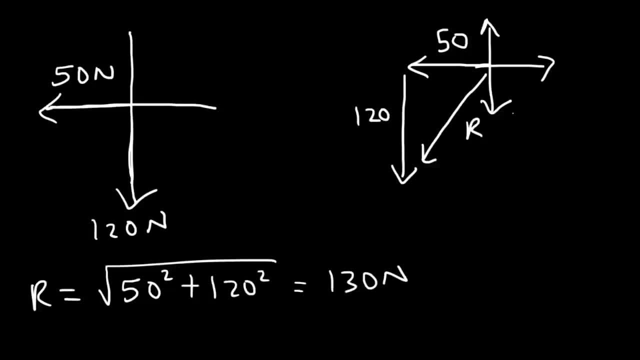 And that's going to turn out to be 130 newtons. So that's the magnitude of the resultant force vector. Now all we need to do is find the angle. So first let's find the reference angle. To find the reference angle, use the arc tangent formula. 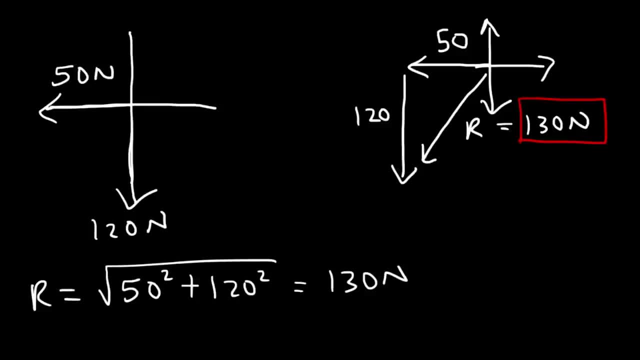 Now all we need to do is find the angle. So first let's find the reference angle. To find the reference angle, use the arc tangent formula. take the force in the y-direction divided by that in the x-direction, But make it positive initially. 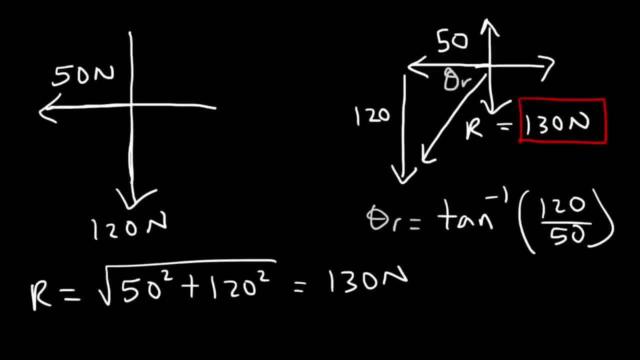 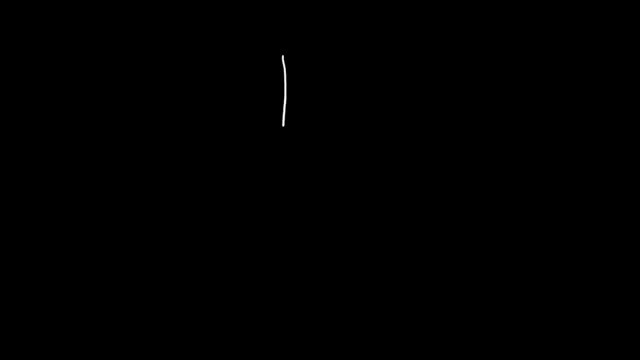 This will give you an acute angle between 0 and 90.. And then you can address it later. So arc tan 120 over 50 will give you a reference angle of 67.4.. So here's the reference angle. It's inside the triangle. 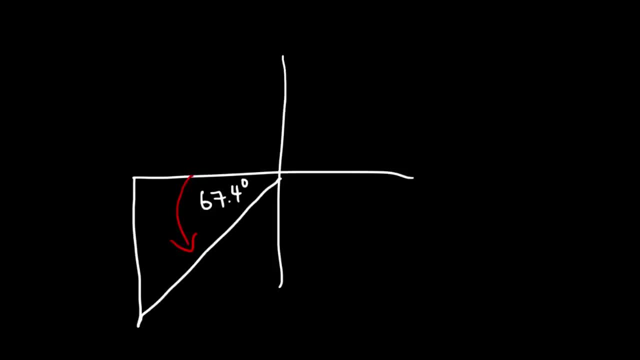 Now what we need is the angle relative to the positive x-axis. So if this is 180, then the resultant vector is 180 plus 67.4 relative to the x-axis, So it's at an angle of 247.4.. 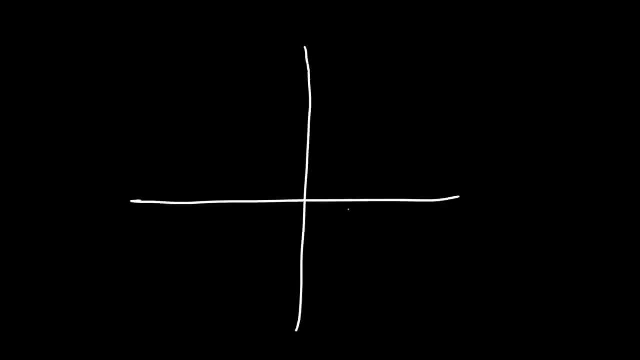 So therefore, this is the resultant force vector, which has a magnitude of 130, but an angle of 247.4 degrees. So that's the answer. Now, let's say, if we have a force vector of 45 newtons directed east, 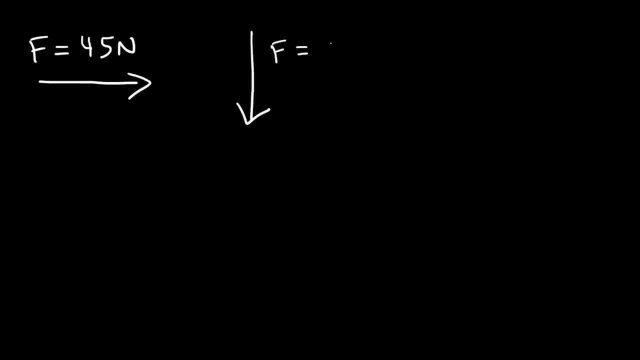 and we wish to add it to a force vector of 60 newtons directed south. Find the magnitude of the resultant force vector and also the angle. So let's draw a triangle. So this is 45, and this is 60.. 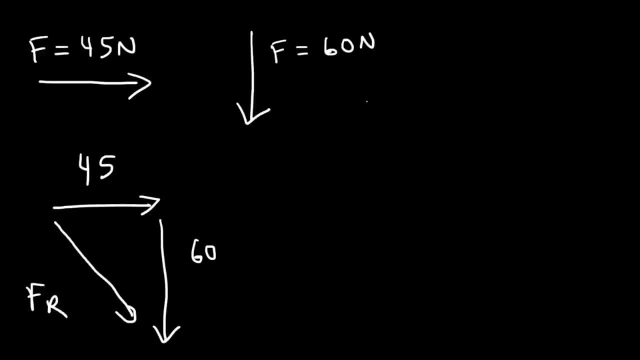 So let's find the magnitude of the resultant force vector. So it's going to be the square root of 45 squared plus 60 squared, Which is 75 newtons. So that's the magnitude. Now we've got to find the angle. 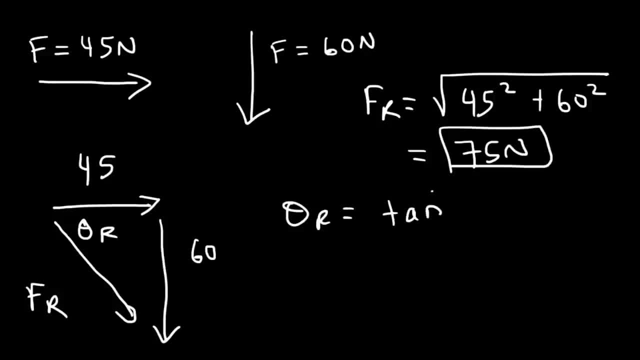 But let's find a reference angle first. So it's going to be arc tangent: the force in the y direction divided by the force in the x direction, So that's 60 over 45. Which is 53.1.. Now that's the reference angle. 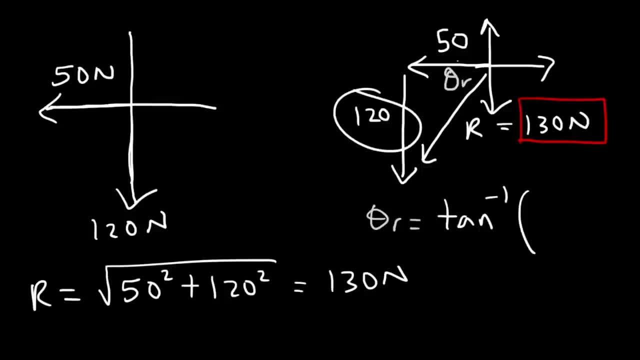 take the force in the y-direction divided by that in the x-direction, But make it positive initially. This will give you an acute angle between 0 and 90. And then you can address it later. So arc tan 120 over 50 will give you a reference angle of 67.4.. 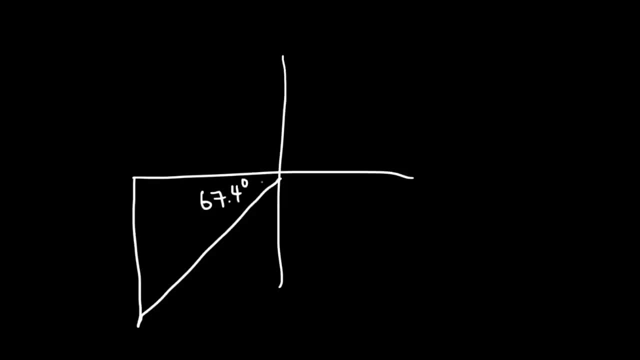 So here's the reference angle. It's inside the triangle. Now what we need is the angle relative to the positive x-axis. So if this is 180, then the resultant vector is 180 plus 67.4 relative to the x-axis. 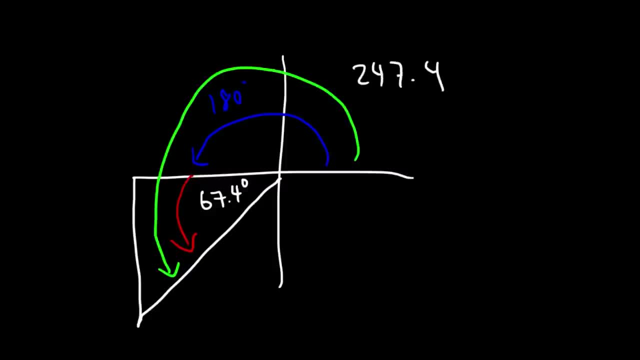 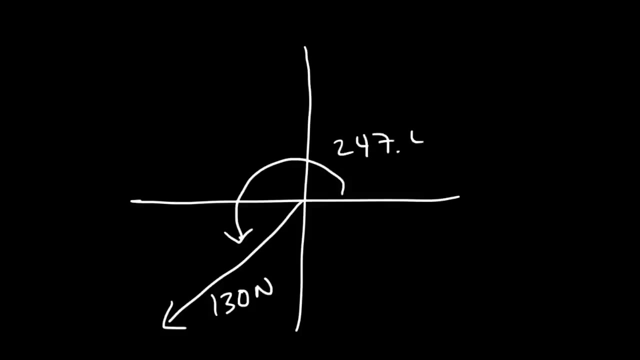 So it's at an angle of 247.4.. So therefore, this is the resultant force vector, which has a magnitude of 130, but an angle of 247.4 degrees. So that's the answer. Now let's say, if we have a force vector of 45 newtons directed east, 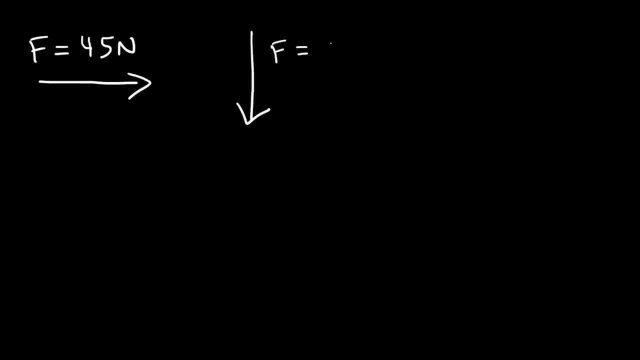 and we wish to add it to a force vector of 60 newtons directed south. Find the magnitude of the resultant force vector and also the angle. So let's draw a triangle. So this is 45, and this is 60.. 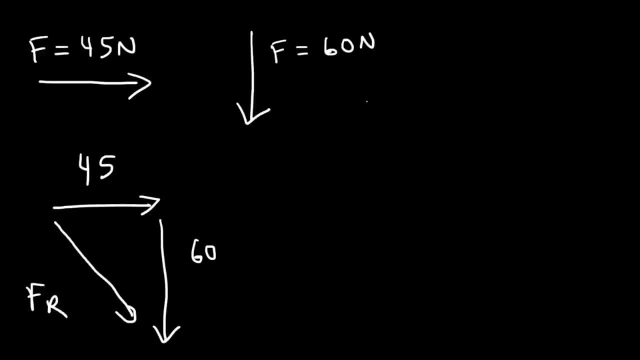 So let's find the magnitude of the resultant force vector. So it's going to be the square root of 45 squared plus 60 squared, Which is 75 newtons. So that's the magnitude. Now we've got to find the angle. 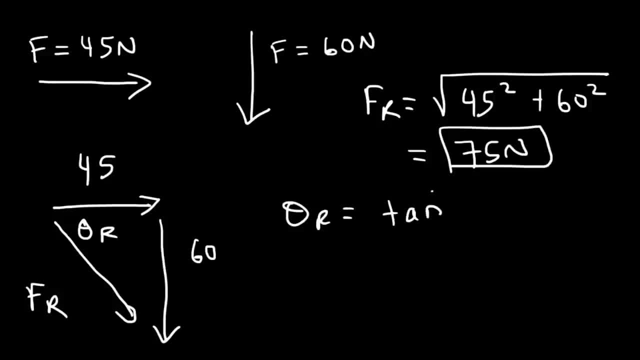 But let's find a reference angle first. So it's going to be arc tangent: the force in the y direction divided by the force in the x direction, So that's 60 over 45. Which is 53.1.. Now that's the reference angle. 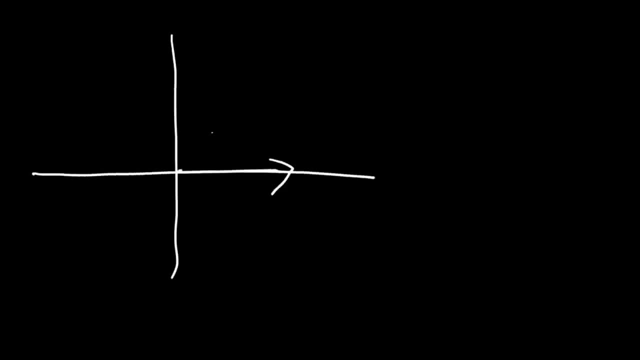 The first force vector is positive, It's directed east. The second one is directed south. So therefore, the resultant force vector is in quadrant 4.. Now, if this angle is 53.1,, to find the angle relative to the positive x axis. 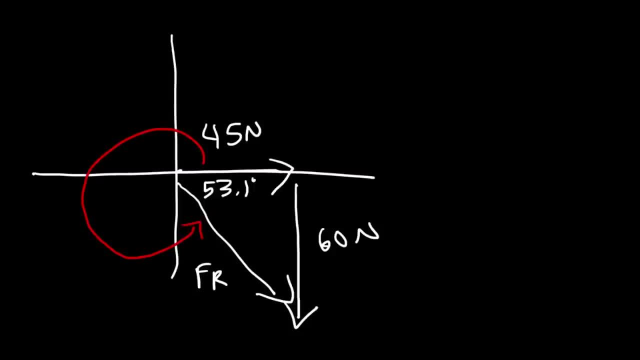 it's going to be 360 minus 53.1.. Keep in mind, a full circle is 360.. But you need to go back 53.1 degrees. So 360 minus 53.1 will give us an angle of 306.9.. 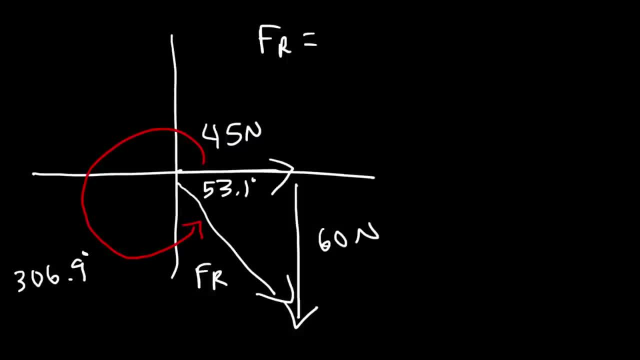 So the resultant force vector has a magnitude of 75 newtons and it's directed at an angle of 306.9 degrees relative to the positive x axis. So this is the answer. So, if you know, the resultant force vector is going to be in quadrant 1,. 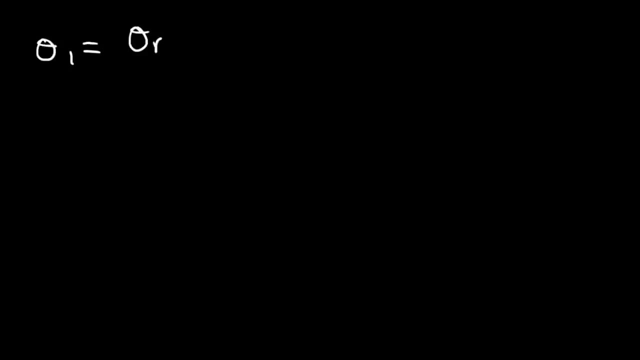 then the angle is going to be the same as the reference angle. And keep in mind, the reference angle can be calculated by taking the inverse tangent of the force in the y direction divided by the force in the x direction. And if you always make these positive, 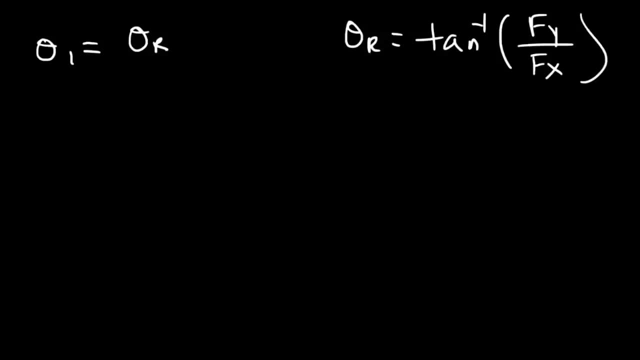 you're always going to get an acute angle between 0 and 90, which is the reference angle. Now, if you know the resultant force vector is in quadrant 2, then to find that angle, it's going to be 180 minus the reference angle. 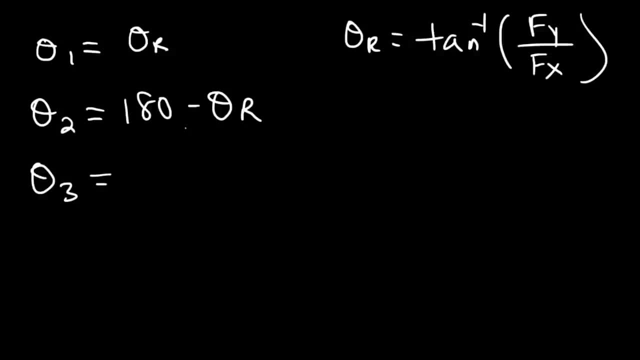 If it's in quadrant 3, we covered this one already- it's 180 plus the reference angle. And if you get an answer that's in quadrant 4, it's going to be 360 minus the reference angle, which was the case in the last example. 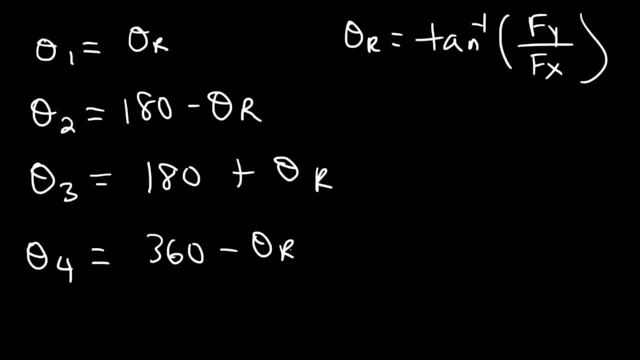 So it's helpful to know these things, or you could just see what to do visually once you graph everything. Now, sometimes you may need to add vectors that are not parallel or perpendicular to each other. So let's say, if we want to add this vector, 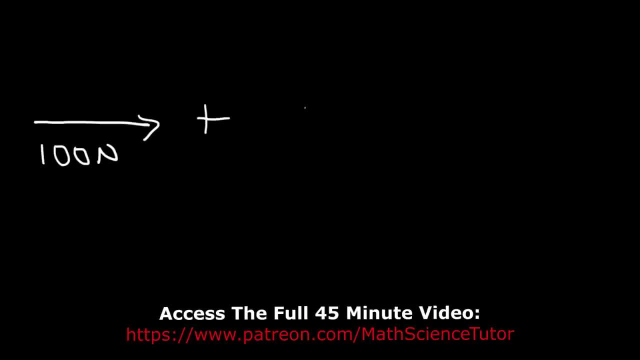 which is 100 newts directed east, plus another vector. let's say it has a magnitude of 150, but it's directed at 30 degrees above the x axis. How can we find the resultant vector? First, let's relist what we have. 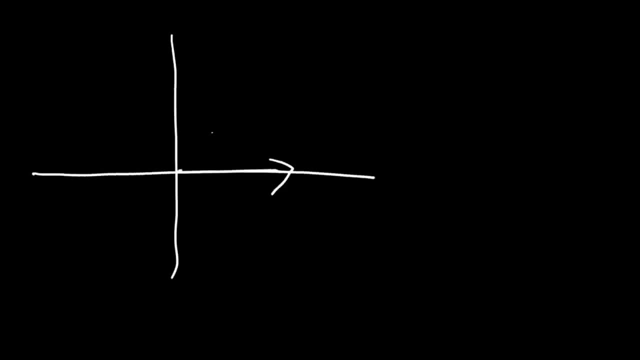 The first force vector is positive, It's directed east. The second one is directed south. So therefore, the resultant force vector is in quadrant 4.. Now, if this angle is 53.1,, to find the angle relative to the positive x axis. 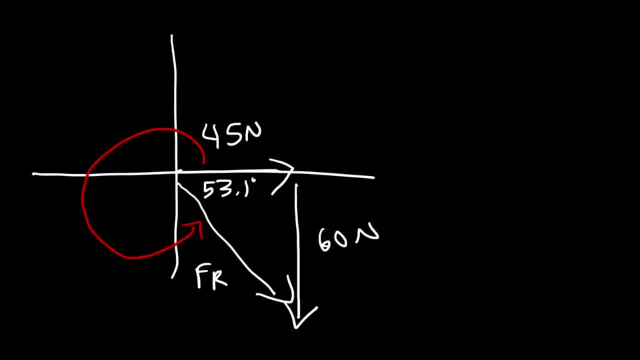 it's going to be 360 minus 53.1.. Keep in mind, a full circle is 360.. But you need to go back 53.1 degrees. So 360 minus 53.1 will give us an angle of 306.9.. 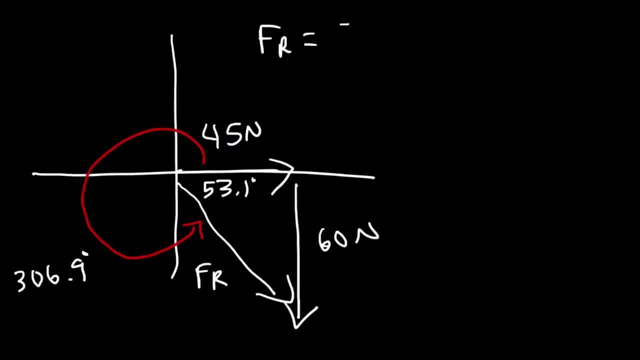 So the resultant force vector has a magnitude of 75 newtons and it's directed at an angle of 306.9 degrees relative to the positive x axis. So this is the answer. So, if you know, the resultant force vector is going to be in quadrant 1,. 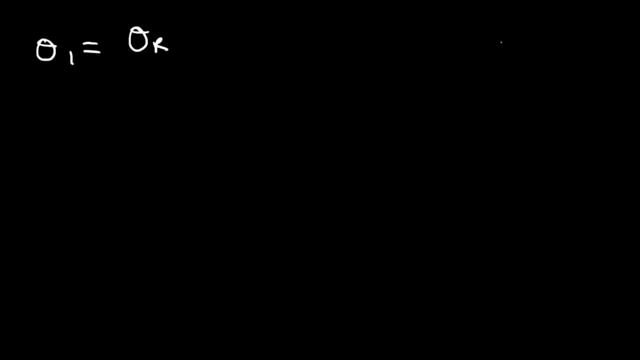 then the angle is going to be the same as the reference angle. And keep in mind, the reference angle can be calculated by taking the inverse tangent of the force in the y direction divided by the force in the x direction. And if you always make these positive, you're always going to get an acute angle between 0 and 90, which is the reference angle. 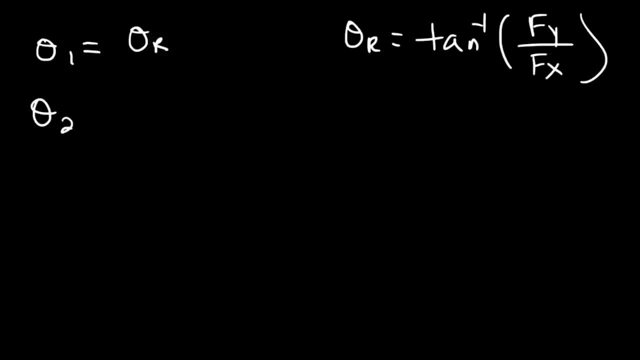 Now, if you know the resultant force vector is in quadrant 2, then to find that angle, it's going to be 180 minus the reference angle. If it's in quadrant 3, we covered this one already- it's 180 plus the reference angle. 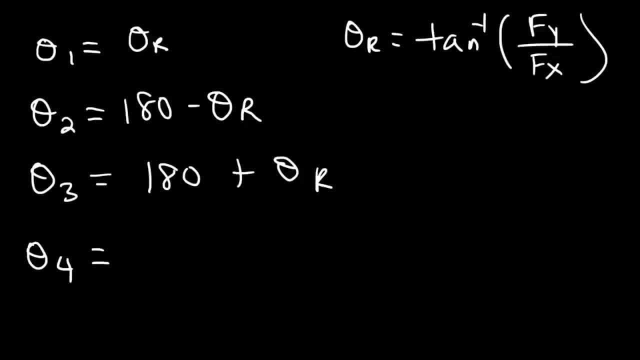 And if you get an answer that's in quadrant 4, it's going to be 360 minus the reference angle, which was the case in the last example. So it's helpful to know these things, or you could just see what to do visually once you graph everything. 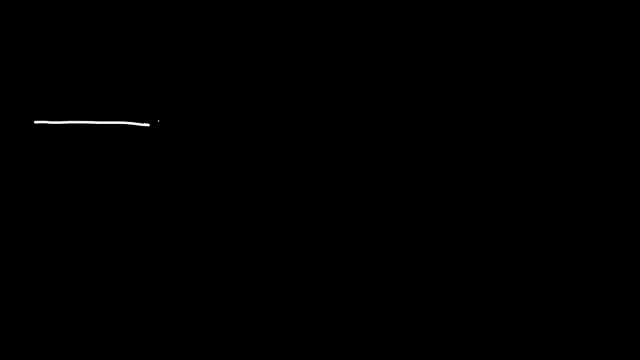 Now, sometimes you may need to add vectors. So here's an example. So you may need to add vectors that are not parallel or perpendicular to each other. So let's say, if we want to add this vector, which is 100 newt-inch directed east, plus another vector, 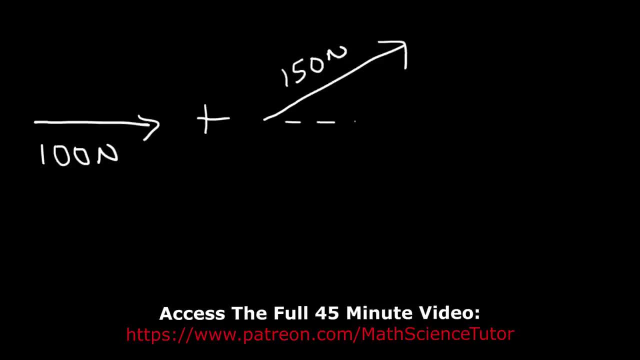 Let's say it has a magnitude of 150, but it's directed at 30 degrees above the x-axis. How can we find the resultant vector? First, let's relist what we have. The first vector has a force of 100 newtons. 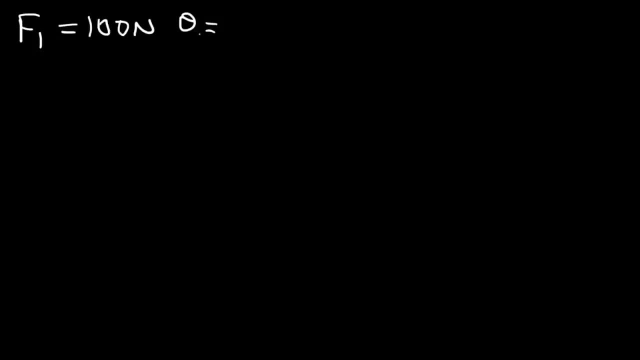 and its angle. it's east, so it's on the x-axis, so it has an angle of 0 degrees. The second force vector has a magnitude of 150 newtons and it has an angle of 30 degrees relative to the x-axis. 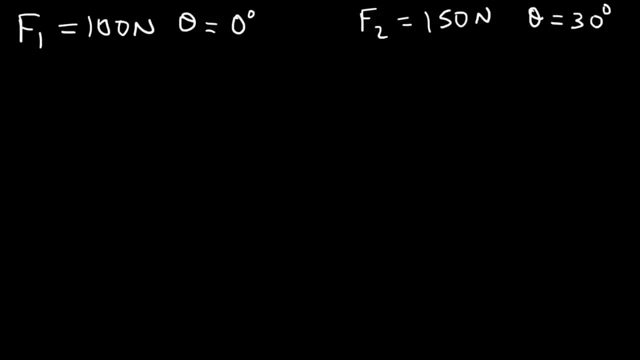 Now what you want to do is you want to add these vectors using the component method. You want to break these forces into their components, add their respective x and y components, and then you can find the resultant force vector. So let's say, if this is a force vector, this is the x component and this is the y component. 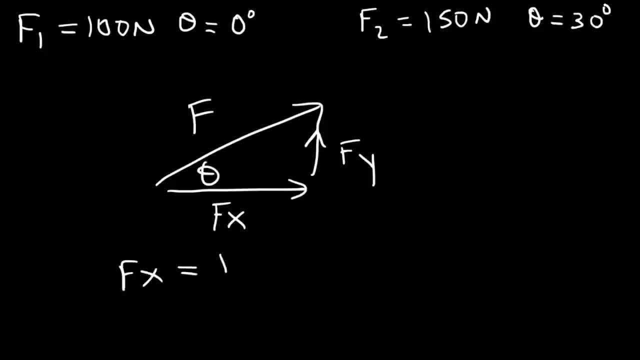 And here is the angle: f of x is equal to f cosine theta and f of y is f sine theta f. you can find it by using Pythagorean Theorem: it's f of x squared plus f of y squared. 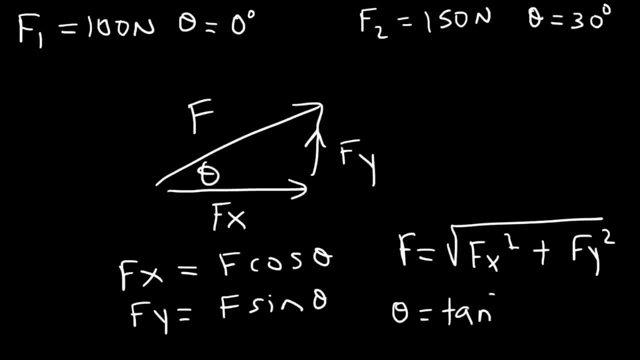 And the angle theta is the arc tangent of f of y divided by f of x. So those are some formulas that you're going to find useful in this portion of the video. So what we need to do is find f1x and f1y. 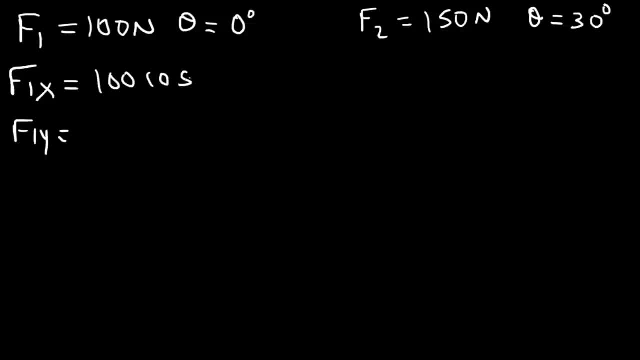 So f1x is going to be 100 cosine of 0.. Cosine of 0 is 1, so 100 times 1 is simply 100.. f1y is going to be 100 sine of 0.. Sine of 0 is 0. 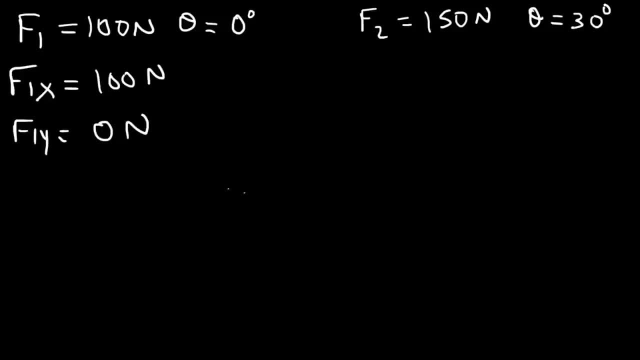 100 times 0 is going to be 0.. Now let's do the same for f2x and f2y. f2x is going to be 0.. Now let's do the same for f2x and f2y. 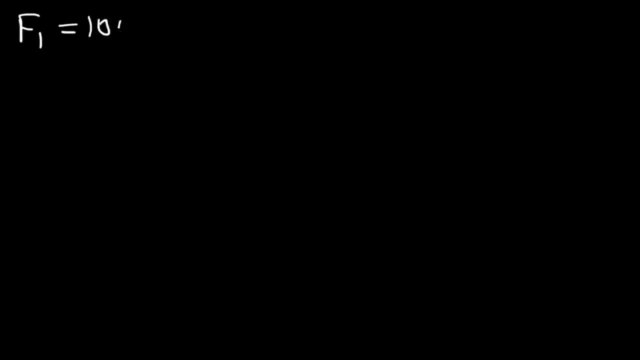 The first vector has a force of 100 newtons and its angle it's east, so it's on the x axis, so it has an angle of 0 degrees. The second force vector has a magnitude of 150 newtons. 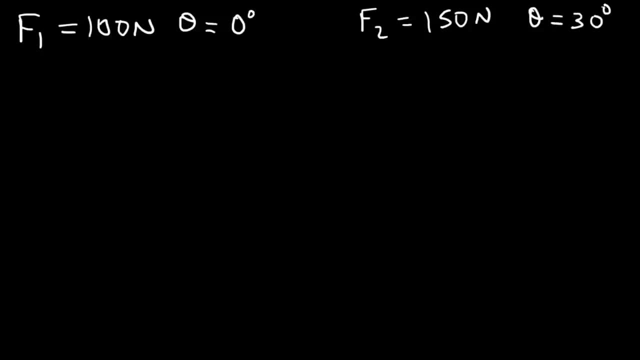 and it has an angle of 30 degrees relative to the x axis. Now what you want to do is you want to add these vectors using the component method. So you want to break these forces into their components, add their respective x and y components. 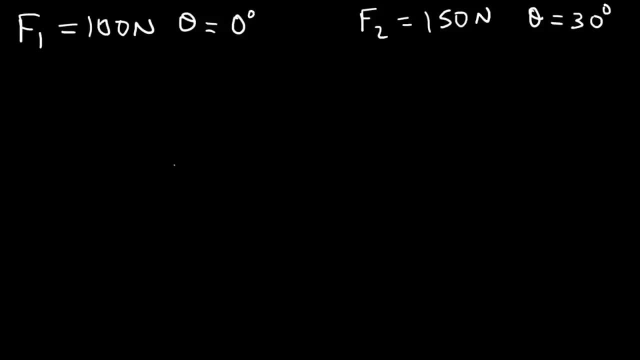 and then you can find the resultant force vector. So let's say, if this is a force vector, this is the x component and this is the y component. And here is the angle: f of x is equal to f cosine theta and f of y is f sine theta. 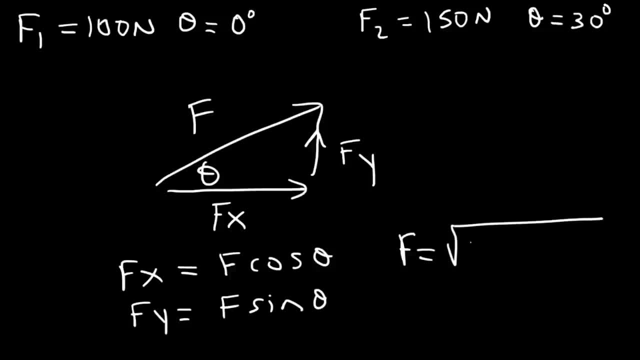 f. you can find it by using Pythagorean theorem. it's f of x squared plus f of y squared, And the angle theta is the arc tangent of f of y divided by f of x. So those are some formulas that you're going to find useful. 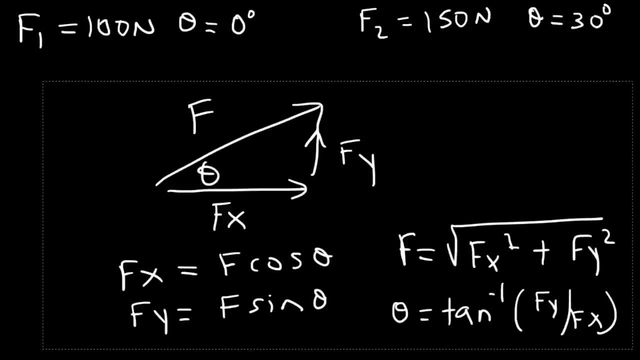 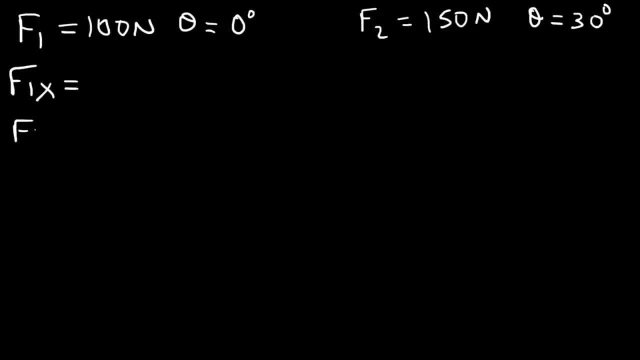 in this portion of the video. So what we need to do is find f1x and f1y. So f1x is going to be 100, cosine of 0.. Cosine of 0 is 1, so 100 times 1 is simply 100. 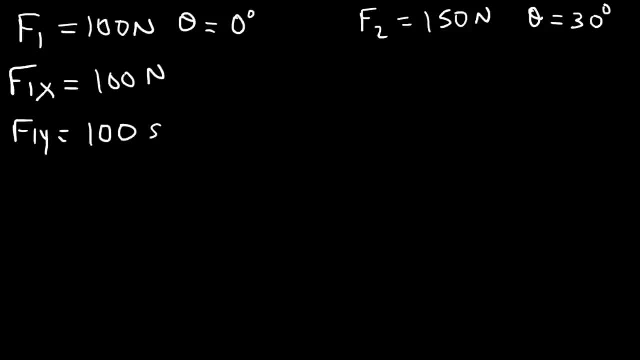 f1y is going to be 100 sine of 0.. Sine of 0 is 0.. 100 times 0 is going to be 0.. Now let's do the same for f2x and f2y. 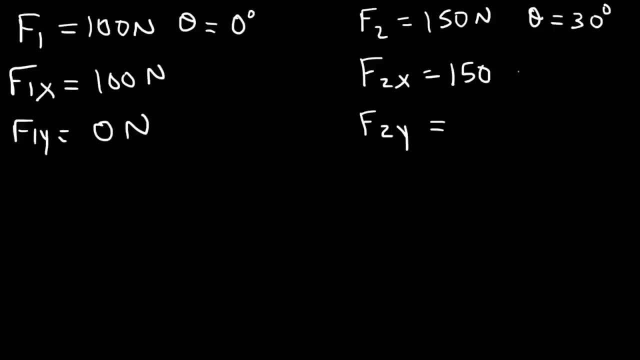 f2x is 150.. times cosine of 30 degrees. Now if you type that in your calculator, make sure it's in degree mode. So this will give you as a decimal, 129.9 newtons. f2y, that's going to be 150 times sine 30,. 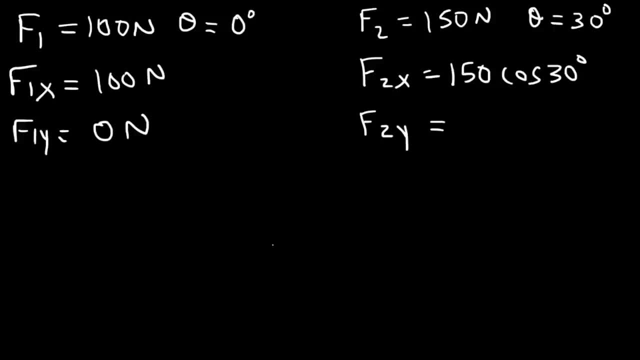 f2x is 150 times cosine of 30 degrees. Now if you type that in your calculator, make sure it's in degree mode. So this will give you as a decimal 129.9 Newtons f2y. that's going to be 150 times sine 30, which is just 75.. 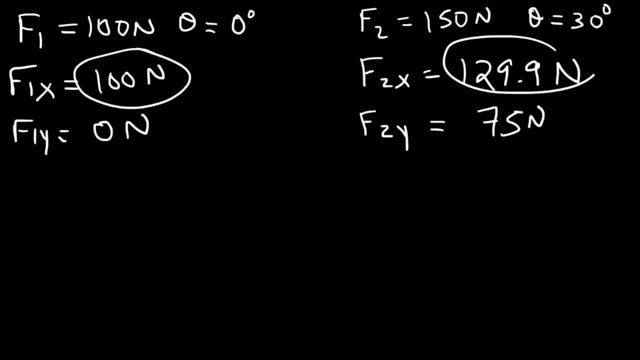 What we need to do is add up the x components. So if we add those two values, the sum of the forces in the x direction is going to be 100 plus 129.9.. So that's going to be 229.9.. 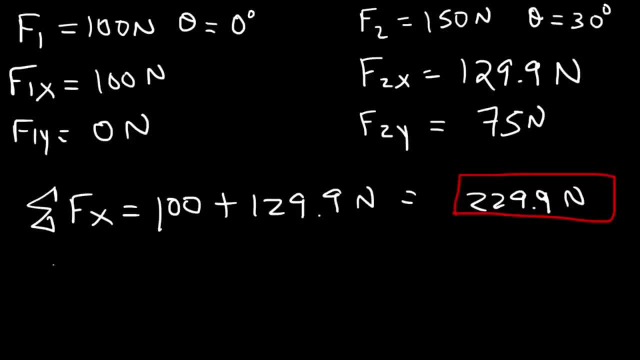 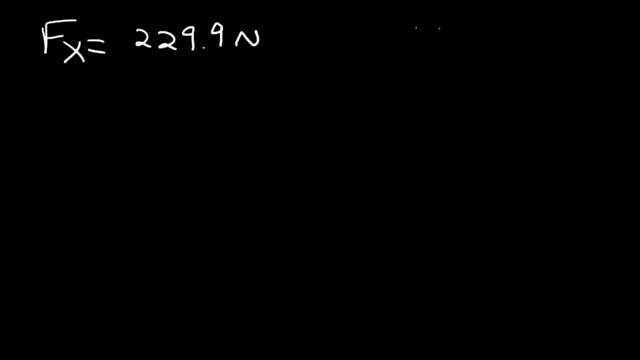 And then we need to find the sum of the forces in the y direction, which is just 0 plus 75. So that's simply 75. So f of x is 229.9 Newtons And f of y is simply 75 Newtons. 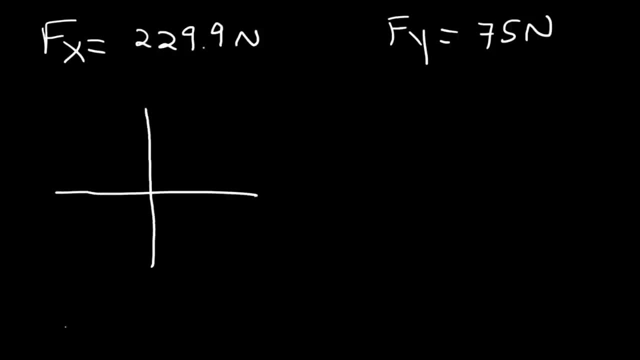 Now let's go ahead and draw these values on an xy plane. So f of x is 229.. And f of y is 75.. The resultant force vector is the hypotenuse And to find it, it's going to be the square root of f of x squared plus f of y squared. 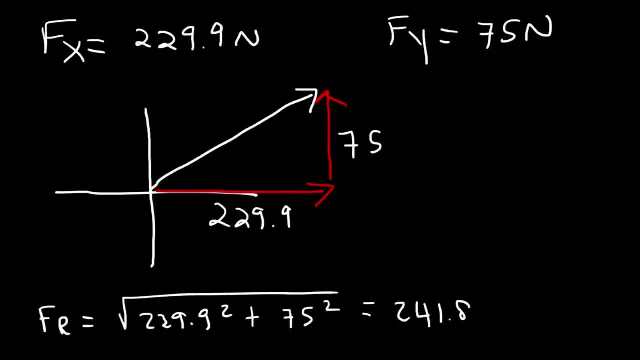 So you should get 241.8.. So that's the resultant force vector. That's the magnitude of it. Now that we have the magnitude, we need to find the angle. So it's going to be arctangent f of y, which is 75,.